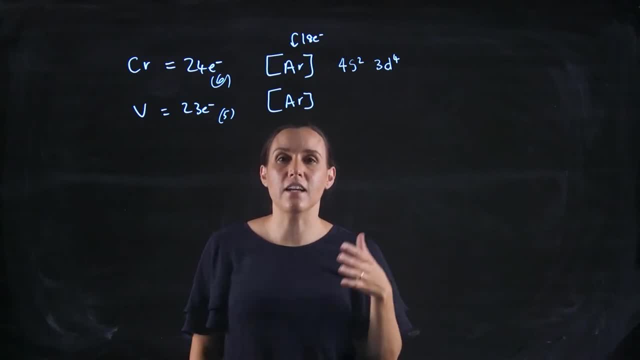 they drop further. So this makes the electrons be promoted from the s block up to the d block, if they can reach those magic numbers. So to half fill them, because there's 5 orbitals, we would be looking at number 5. So a d5 or a d10.. So if we can promote those 2s electrons, 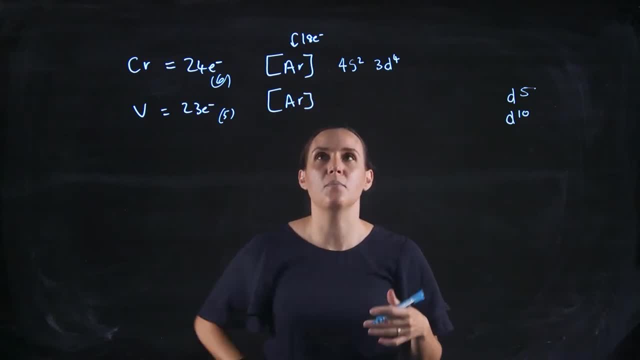 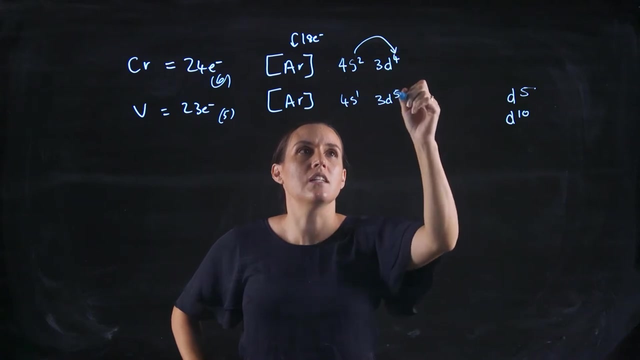 up to the d and hit d5 or d10, that's what's going to happen. So with this one here I could go 4s1, 3d5.. So promote one of these 3d's into the 4, into the 3d, to the 4 to give. 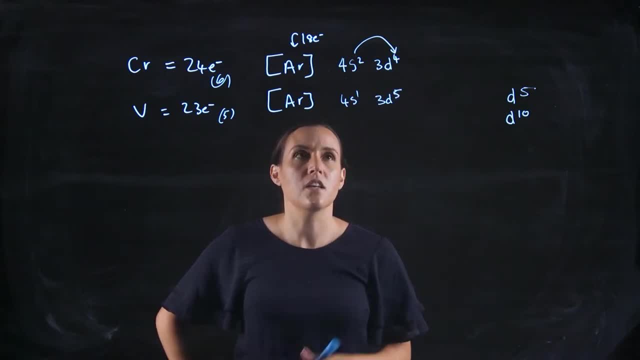 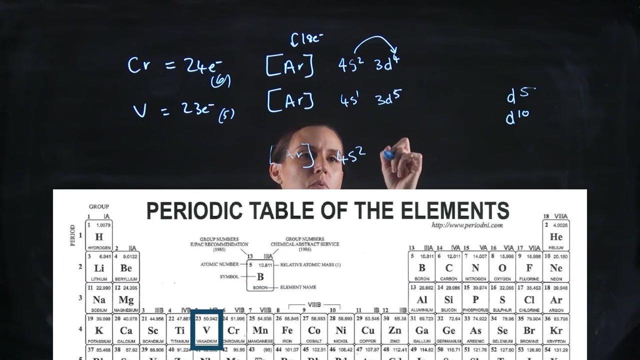 us 5 in that In those orbitals, So that would overall lower the energy of that atom. So for valadium we've got the same. So we've got argon, We've got 4s2.. And I need 5 more electrons So it would. 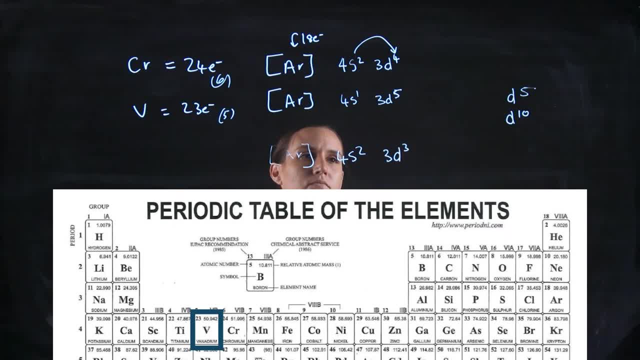 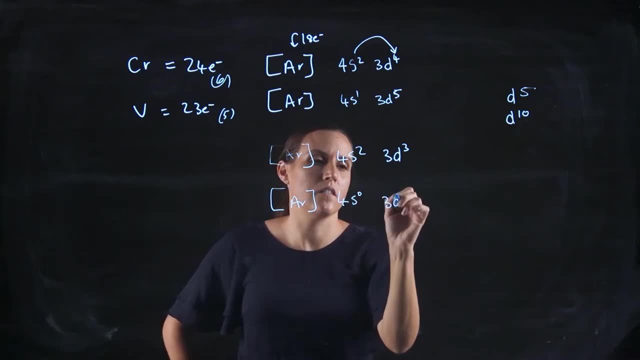 be 3d3.. So 3,, 4, 5.. Now you can see at 3 here I could take 2 from here and reach that magic number of 5.. So that's what the answer would be. So promoting those ones out And that promotion. 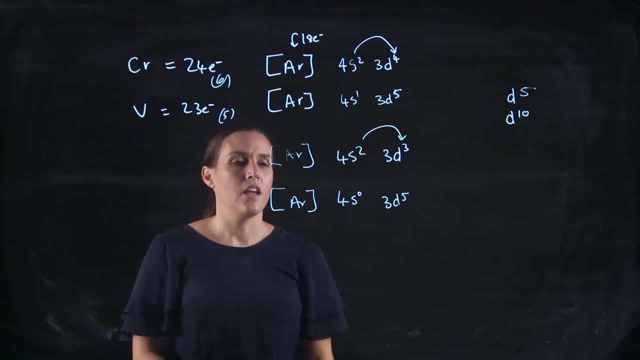 will overall give it a lower energy. Now with the 4s0,, whether or not I write that in, that's optional. Okay, so I don't need to account for that. I could just write argon 3d5. And that would be your answer. 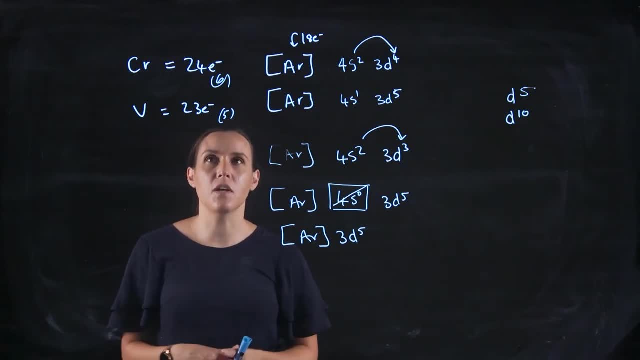 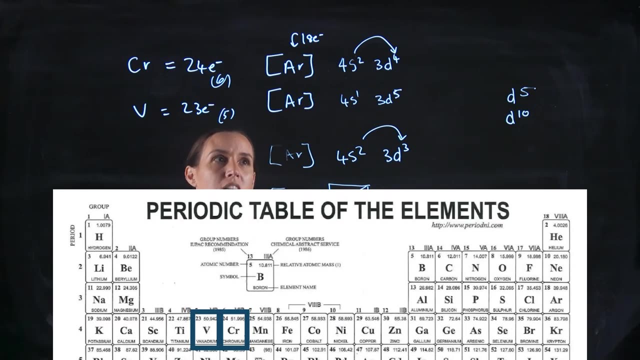 So gives you a bit of ideas about how to do those transition metal ones. so there will be a pattern. so anything that's got 3d4, that will promote one up, anything that's got 3d3 that will promote two up, so it will be the 4d4, the 4d3. 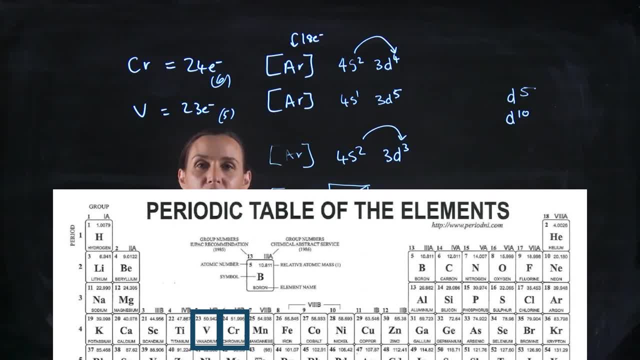 would do the same. and then when you're getting to that magic number of ten. so if it's got d8, it's going to take two, if it's got d9 is going to take one to reach that number ten. so promoting from the s up to the D to give it an overall.